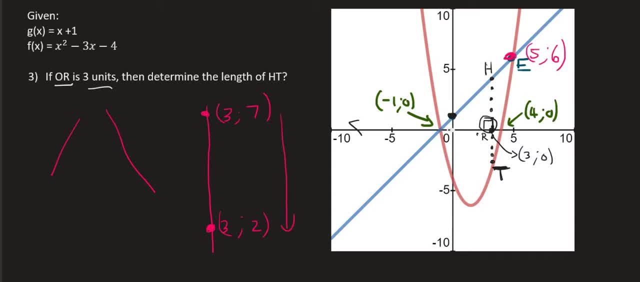 and this y value might be two. then what would this length be? Well, that length would be five, because seven minus two is five. Notice, we don't need to use the distance formula, because the distance formula only needs to be used if we have a diagonal line, But if it's, 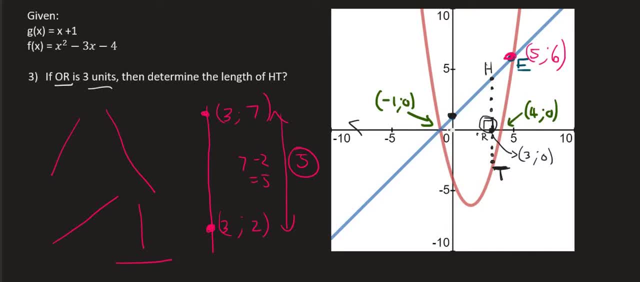 vertical or horizontal. you can just minus the two values. What we can say then is that if the x value of R is three, then that means that the x value at H is also three. So I'm just going to write that over here: So if the x value at H is three, then that means that the x value at H is. 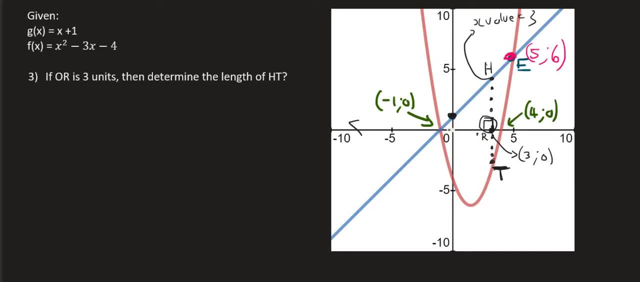 three, and the x value at T is also going to be three. So we know that H is on the straight line. So if we want to know what the y value is at that point, we can just plug the x value into. 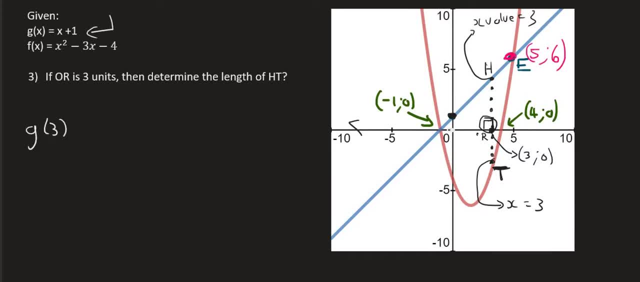 the straight lines equation. So we can plug in three into the place of x and that's going to give us a y value of four. So the y value of H is four. Then we can plug a x value of three into. 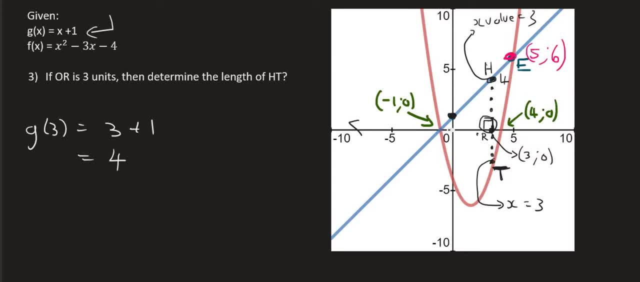 the parabola's equation for T, because T is on the parabola. So that will say f of three equals to three squared minus three times three. Notice I use a bracket and that's going to give us nine minus nine minus four, and that's going to give us minus four. Okay, so the y value of T is minus. 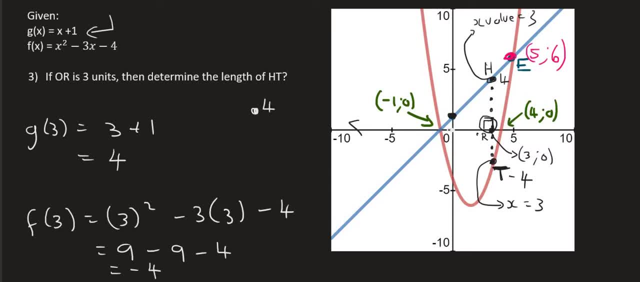 four. So if you have a y value of four and another y value of minus four, then what is that distance? Well, it's eight, because it's four minus minus four, which is eight. So the length of H T will be eight units. 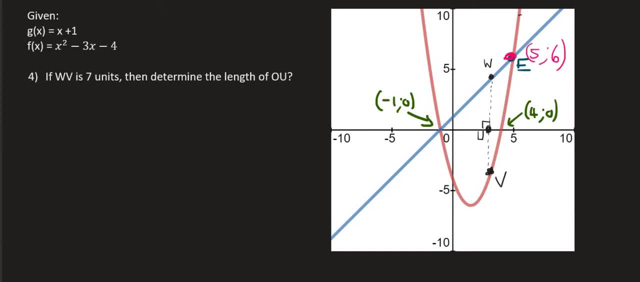 Now here's another way that they can ask this question. Now, this one's similar to what we've just done, but they ask it in a different way. So in the previous question that we just did, I'm just going to quickly draw this over here- In the previous question, they gave you a dotted line. 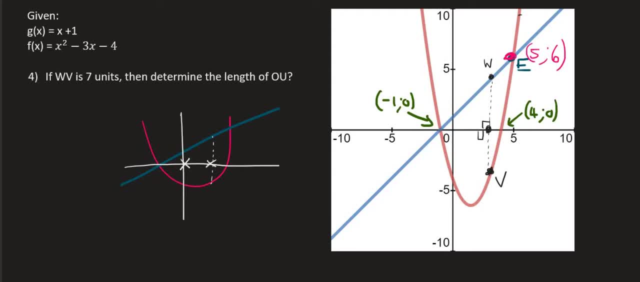 and then what they did is they gave you the length from here to here, So that gave you that was x values, and then you could use this x value over here and you plugged it into this point and this point, and then that allowed you to find this length. Now what we're doing is the. 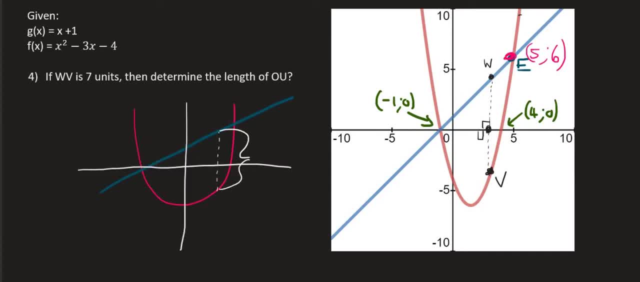 following. Now, what they do is they give you the length first, and then from that you need to work out this. You see, So it's the opposite. In the first one, we gave you the x first, and then you. 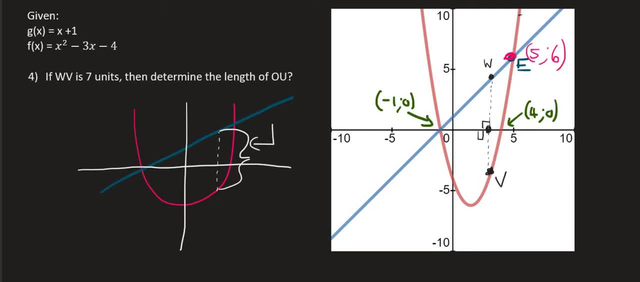 found the y values. Now they're giving you the y value first and you need to find x. So how did they work out that length? Well, to get wv, you would have to take the y value of w and you would have had to have. 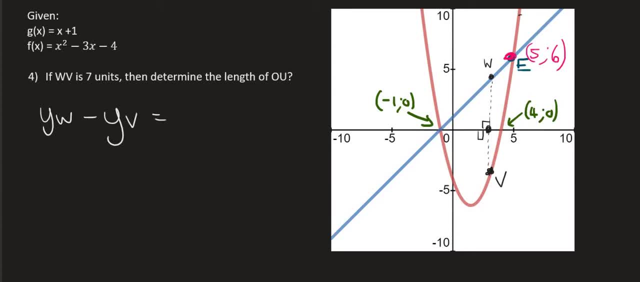 minused it by the y value of v, and that should give you a length of 7.. For example, if wu or uw is 4 units and wv is 3 units, then v's y value would actually be minus 3, right, Because it's. 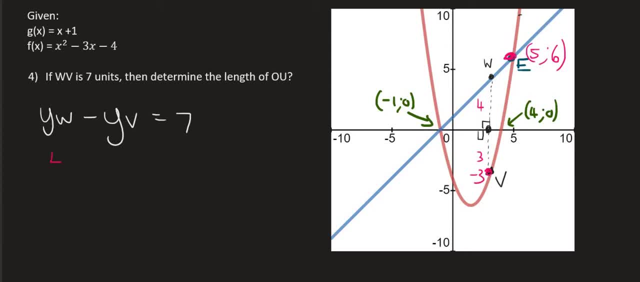 below. So then what you would have said is the y value of w, which is 4,, minus the y value of v, which is minus 3, and then you can see how we would have ended up with 7.. So the main idea is: 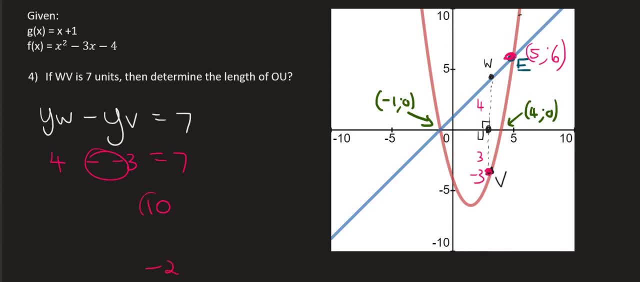 to find the distance between two points, you minus them. Because to get from 10 to minus 2, that's 12, because 10 minus minus 2 is 12.. And it must always be the top one minus the bottom one. 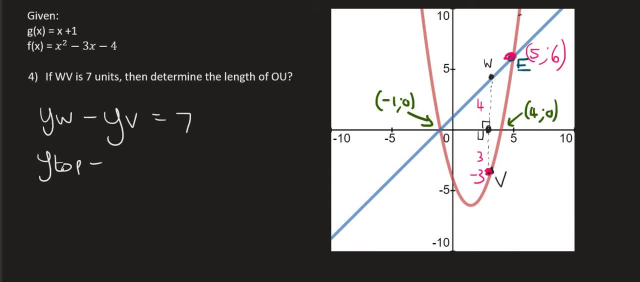 So in a question like this, you might want to remember: y top minus y bottom should give us 7.. But now we can't really do anything else at this point, because what are we looking for? We're looking for the length of ou. Now is ou? does it make you think of the x value or the y values? Well, 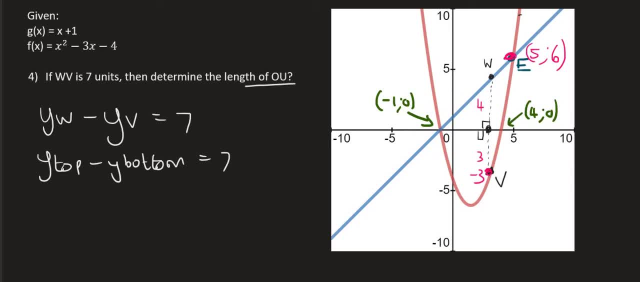 it's the x value. right? If you could get the x value at we need to get the x value at u. So what we do now is we replace these y values over here with x's. Now how do we do that? Well, 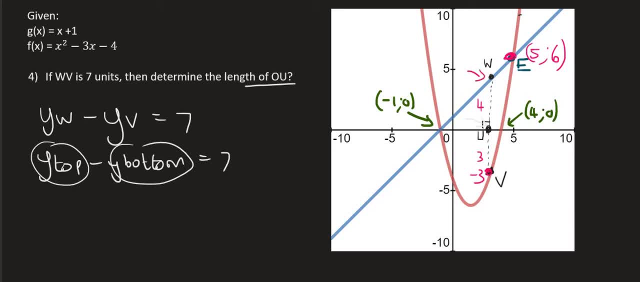 the y value at the top, which is this one over here. that's the straight line, So we can replace this part with its actual equation. So, instead of having it as the y value, you can replace it with x plus 1.. Then you say minus and then you put a bracket. 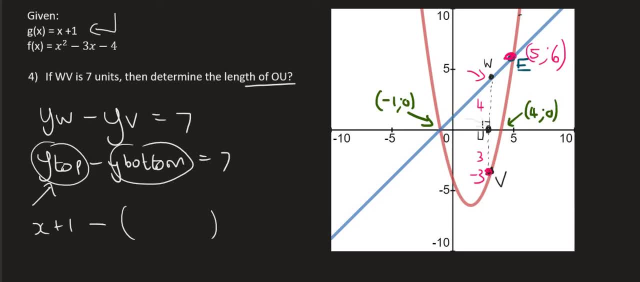 because whenever you minus you should always use a bracket. Then you can replace the y value of the bottom, which is the y value of v, with its equation, which is x squared minus 3x minus 4.. And then you can make that we want that length to be equal to 7.. So now we can just go simplify. 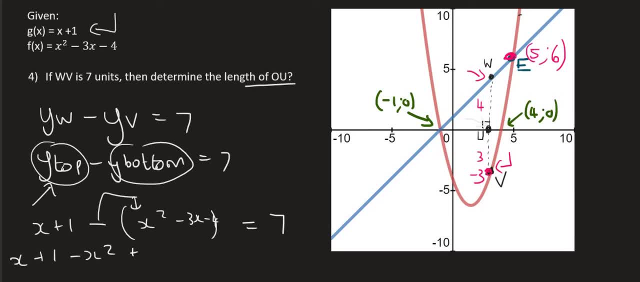 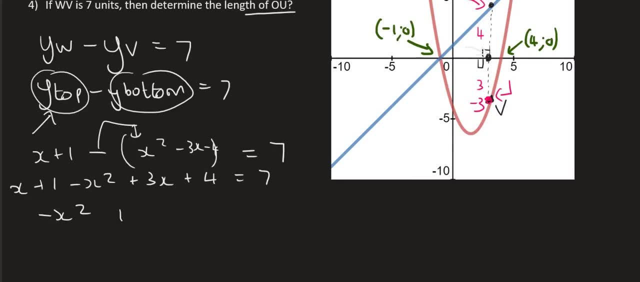 So we put the minus inside the brackets. So it's minus x squared plus 3x plus 4 equals to 7.. Now we just simplify and solve So that'll be negative. x squared plus 4x minus 2 equals to 0.. See what I've done there. The minus 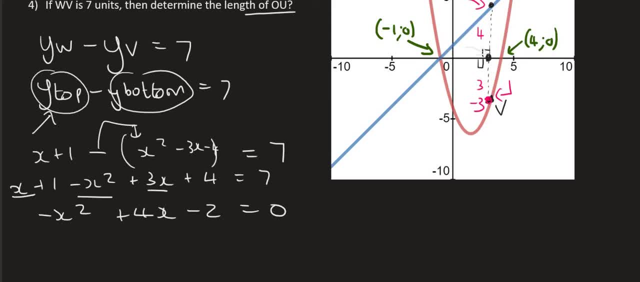 x squared, stays as it is, These two became 4x, and then the 1 and the 4 became 5.. But then, when you bring the 7 over, it becomes minus 2.. You could then solve this however you like You. 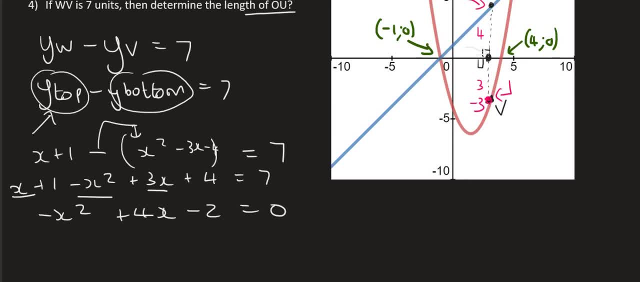 could maybe get rid of the negative. You could factorize. I'm just going to plug it into the formula, which is that one over there, And then I'm going to solve for x, And when you do that, you get two answers, which is very interesting. but I'm going to explain to you what's happening. 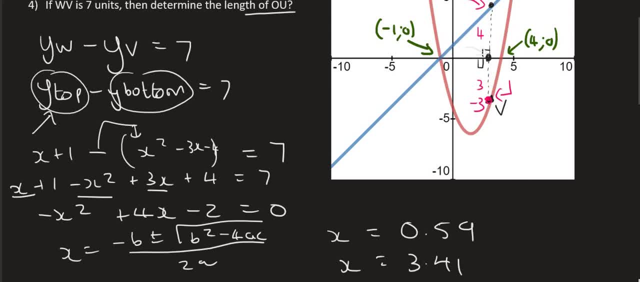 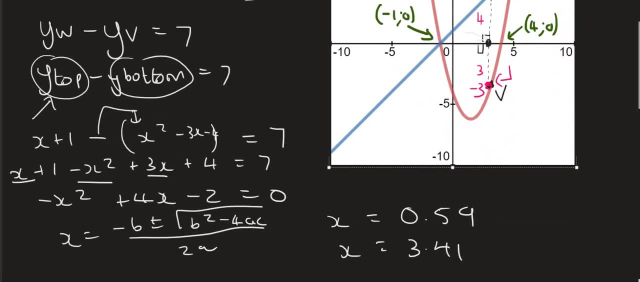 So you get two answers: 0.59 and 3.41.. So what they're trying to tell you there mathematically is that when x is 3.41 or 0.59, then the length between the two graphs is 7.. So 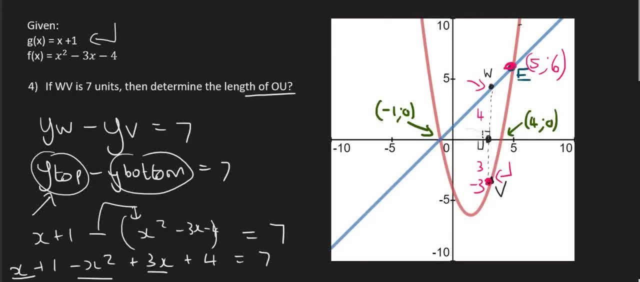 let's see how that works. So if x is 0.51, 0.59, well, that would be somewhere over here maybe, And so we can see that the length between them- they're saying that that length would be 7.. Then if we move a little bit further, 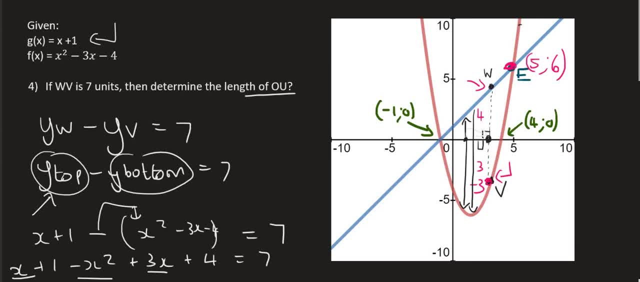 what would happen to the length between the two graphs? Well, it becomes more right, So it's probably like 8 or 9.. But then, as we carry on a little bit further, what happens to the length over there? Well, now the length is becoming slightly smaller, And so there are two places.